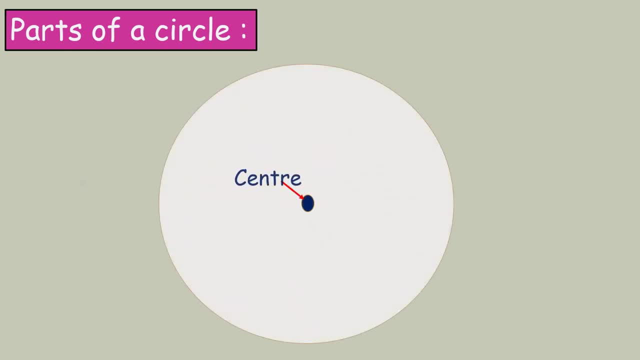 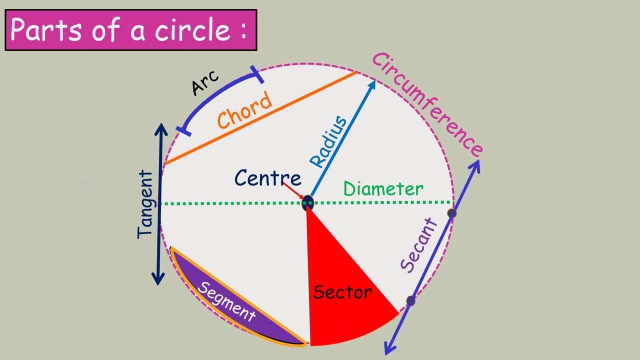 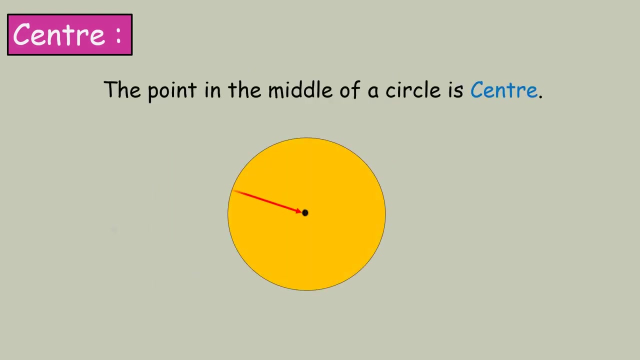 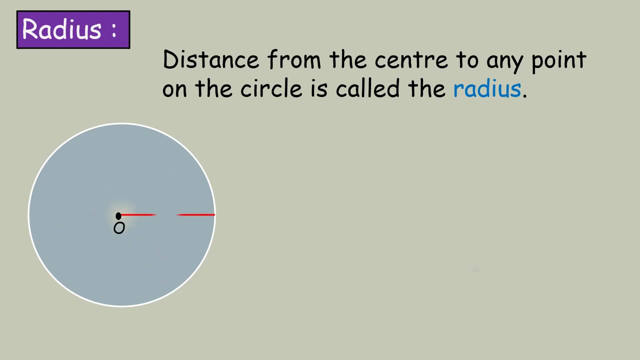 The parts of a circle include center, radius, circumference, diameter, chord, tangent arc, segment, sector and secant. Center is the point in the middle of a circle. Radius is the distance from the center to any point on the circle. 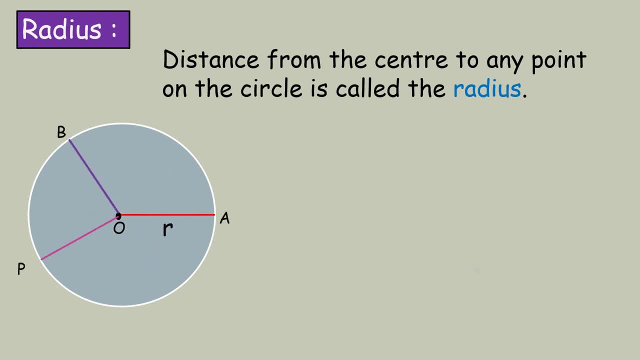 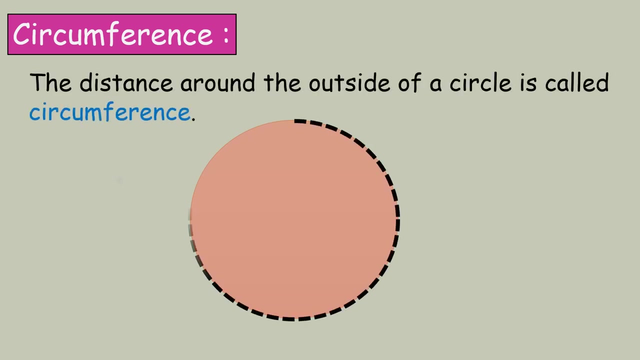 Circle is called the radius. In this circle line, segment OA, OB, OP are the radii of the circle. Here radius is equal to half of the diameter Circumference- The distance around the outside of a circle is called circumference. 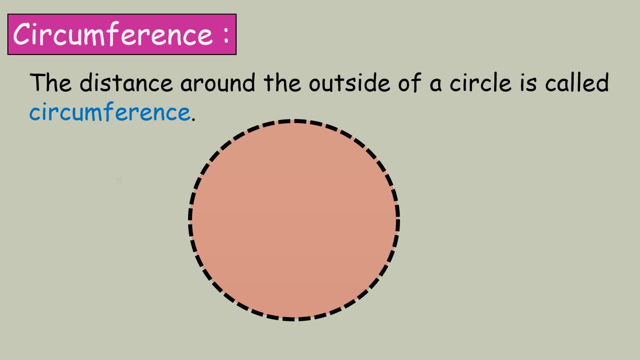 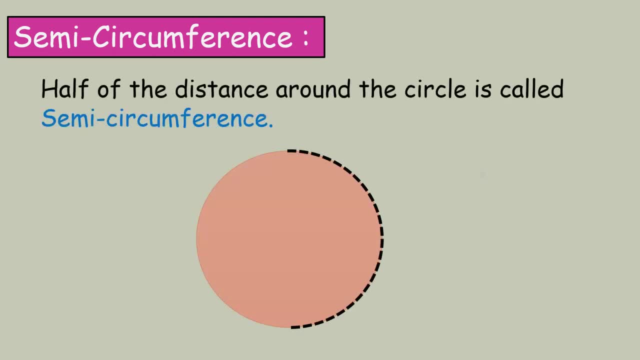 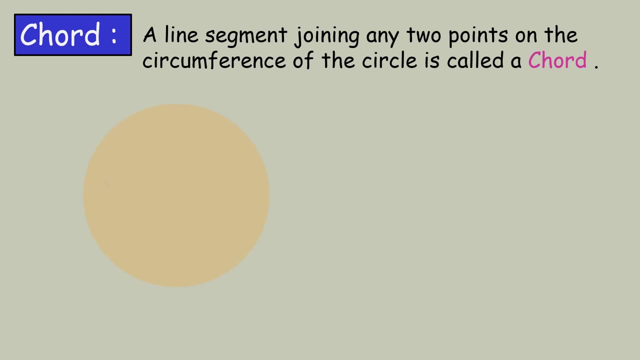 Semicircle, Half of the distance around the circle is called semicircle, Corner, diagonal, half-circle, Semicircle, A line segment joining any two points on the circumference of the circle is called a chord. Here line segment AB, CD, PQ are chords of the circle. 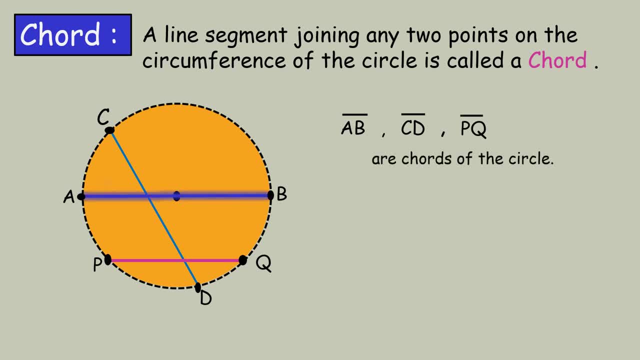 Semicircle: The distance of the circle is equal to half of the distance around the circle. Semicircle: The distance around the circle is called semicircle. The chord AB is the longest chord and it is also the diameter of the circle. 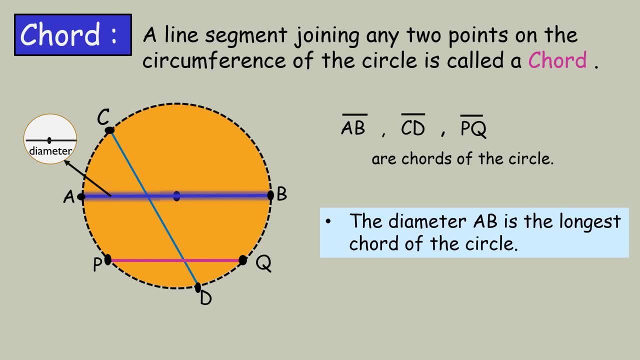 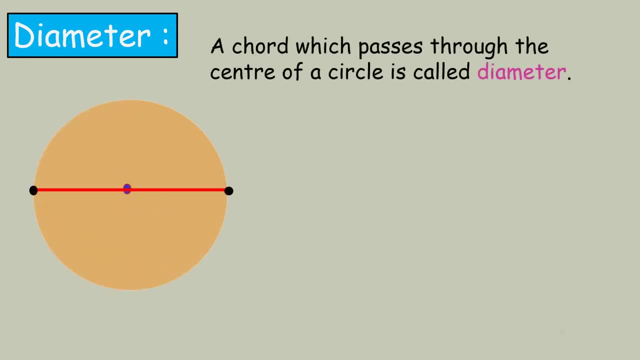 Thus the diameter AB is the longest chord of the circle. Diameter. A chord which passes through the center of a circle is called diameter. Here the diameter of a circle is twice the radius. That is, diameter is equal to 2 into radius. 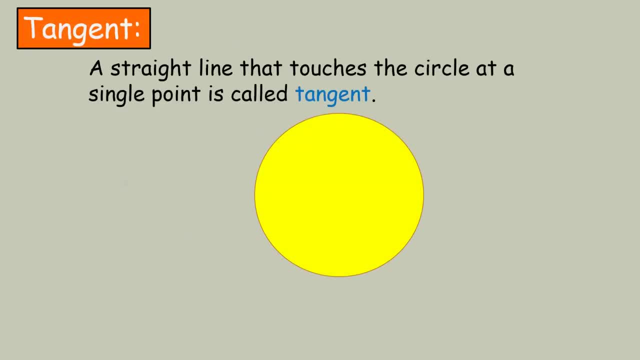 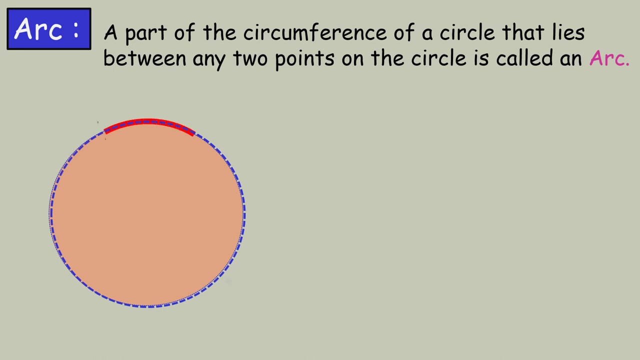 Tangent. A straight line that touches the circle at a single point is called tangent Arc. A part of the circumference of a circle that lies between any two points on the circle is called an arc. It is denoted by the symbol. Here, points P and Q divide the circumference into two arcs.